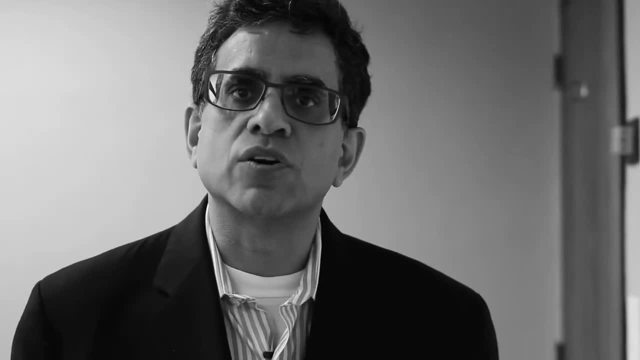 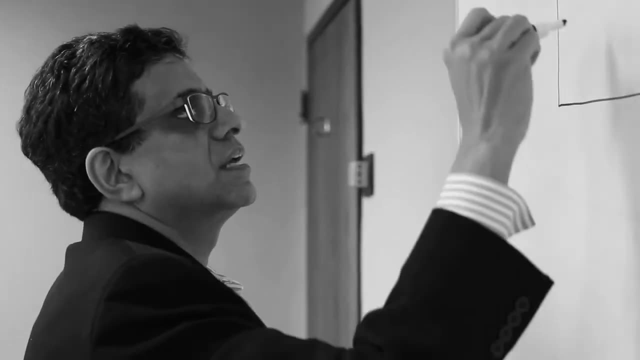 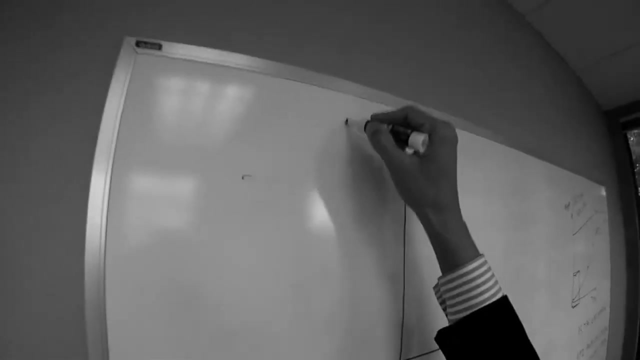 are at different stage in their API strategy and the role that analytics plays in helping them succeed. Let's think about an enterprise as it embarks on its API journey, where we're going to look at the fractional contribution of APIs to the bottom of the API. 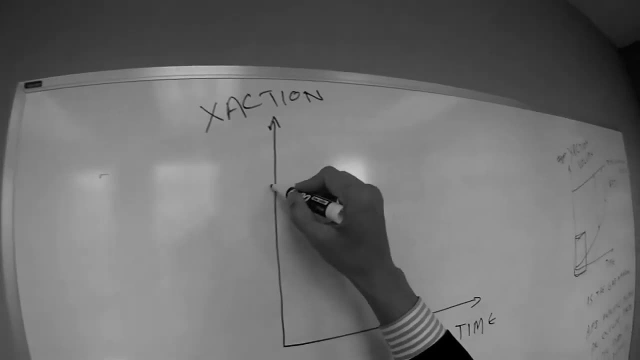 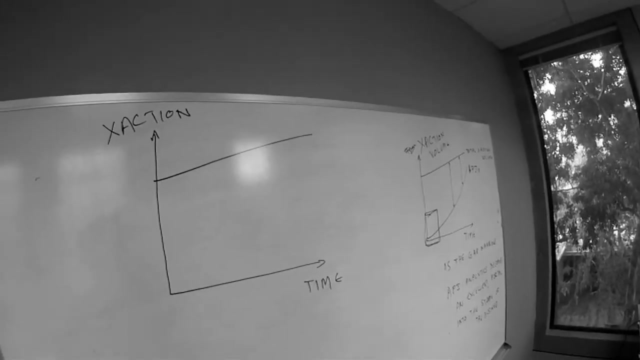 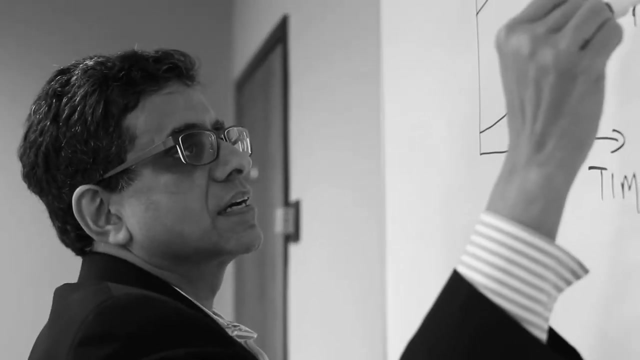 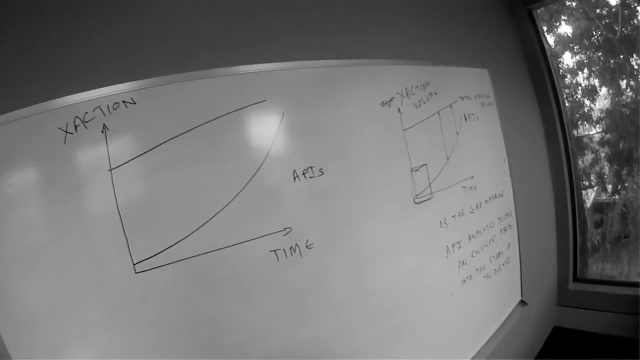 Let's think about an enterprise as it embarks on its API journey, where we're going to look at the fractional contribution of APIs to the bottom of the API. Let's take, for example, a line of the top line and the bottom line of an enterprise. Every enterprise expects to see more transactions, more interactions, more purchases, more buys to happen through their systems, But in fact, the API delivered transactions are. 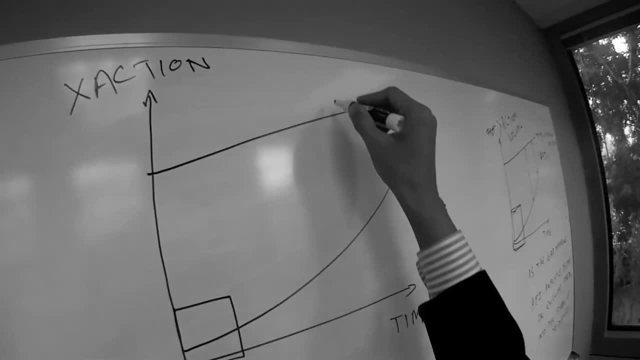 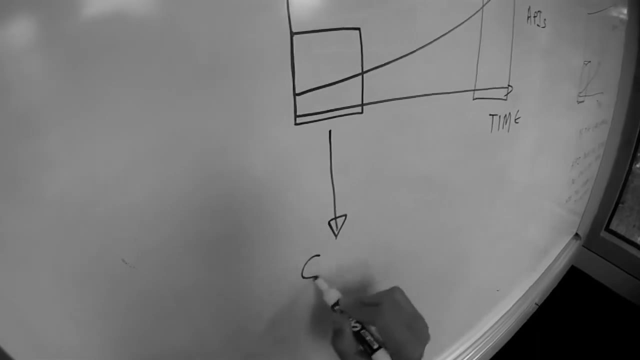 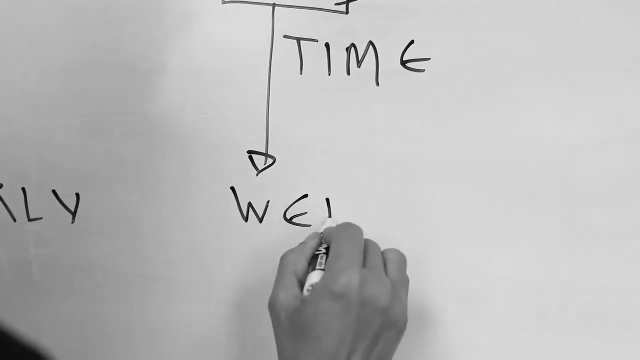 going to contribute an increasingly larger fraction to this bottom line or top line, And what we're going do is we are going to examine two companies: a company that is just embarking on its API strategy and a company that is well into its API strategy. as an example of the former, think about a company that has built out. 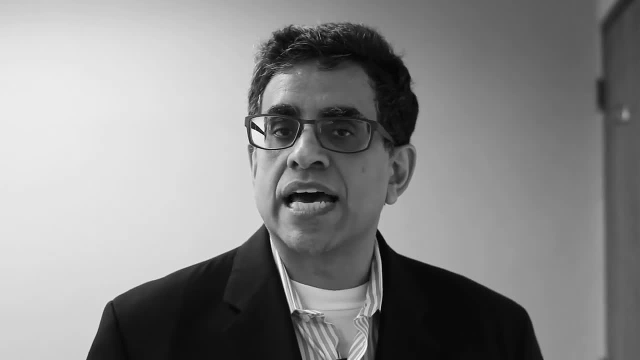 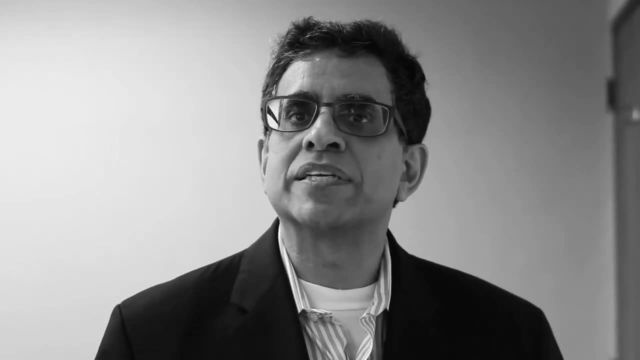 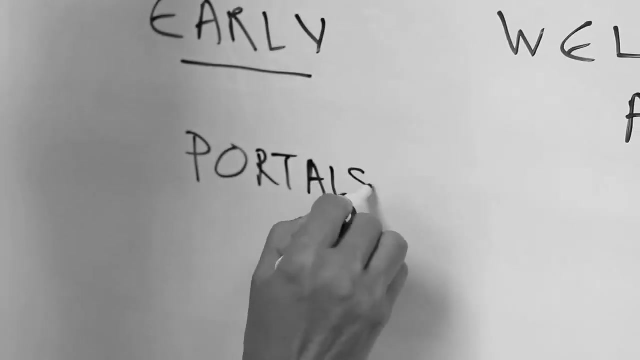 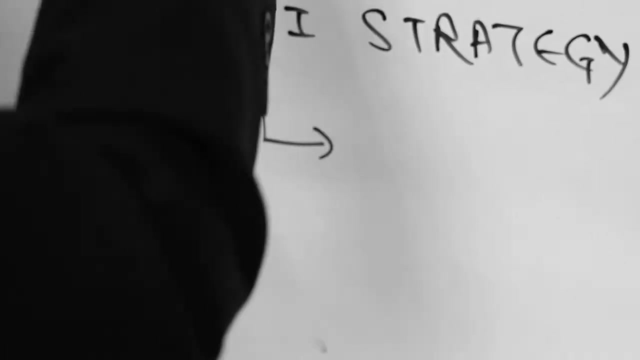 a sass application and now it realizes that, as it is attracting more and more enterprise-class customers, it needs to open up its sass applications through API. they go from portal to API. as an example of a late-stage company or a company where API is contribute a large fraction to the transaction, think about: 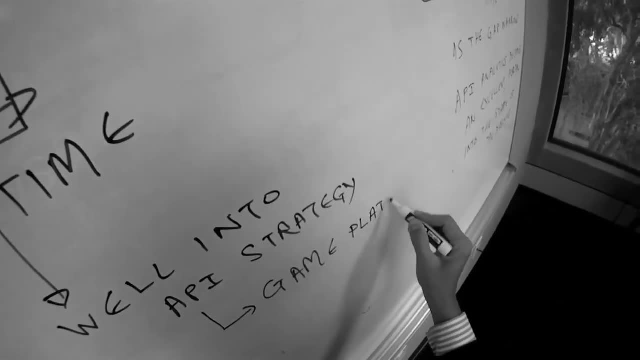 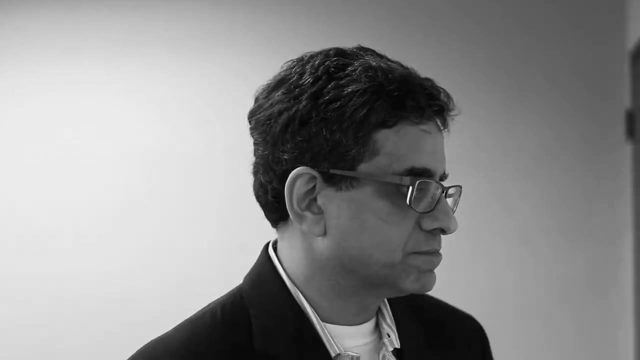 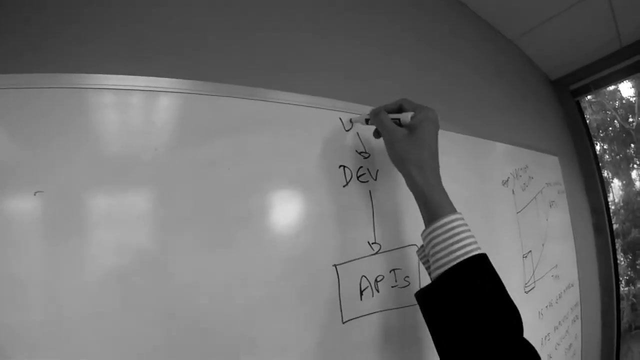 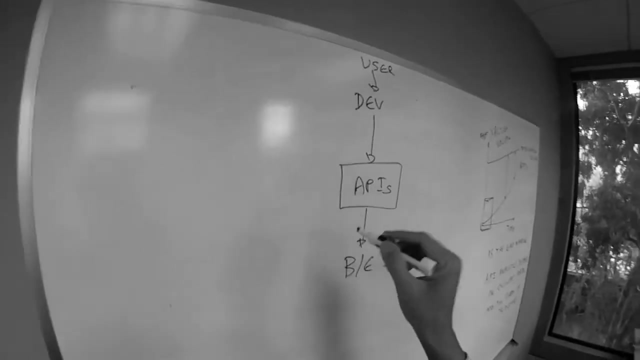 a guy game platform where APIs represent the bulk of the traffic that happens within that particular enterprise. So let's first take a look at the early stage. So APIs, as we have discussed, connect developers, users, developers to back-end systems. Analytics on those APIs helps many constituents. 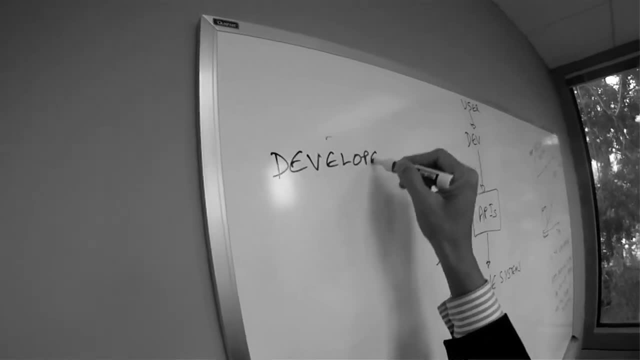 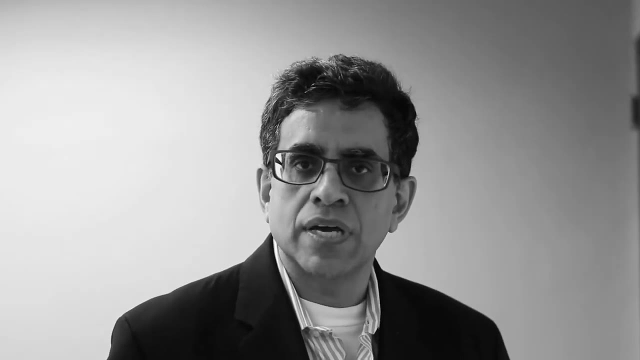 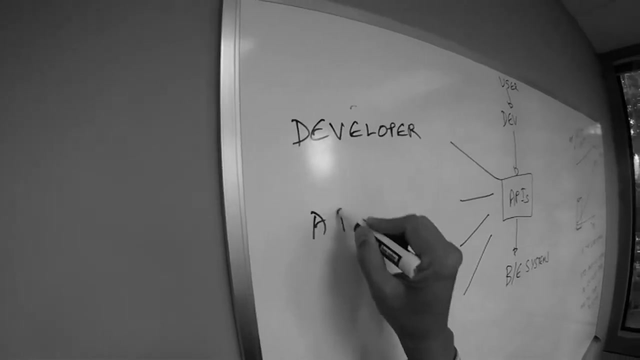 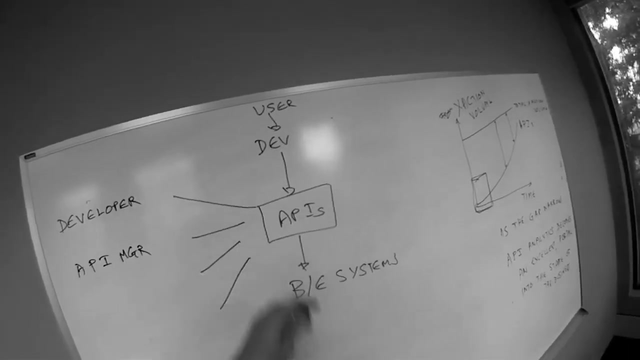 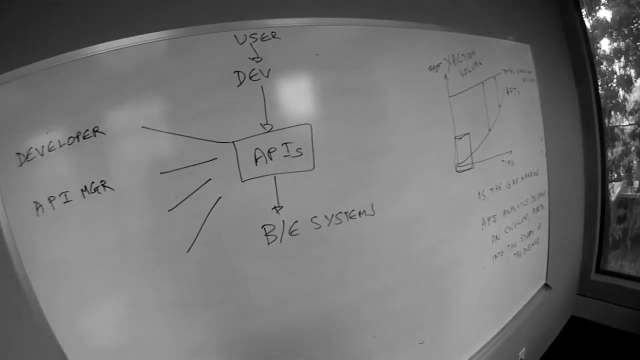 The developer will benefit by understanding how much is he contributing to the bottom line of that enterprise and that may help him actually get better deals out of that particular enterprise. If I am the API manager responsible for the success of those APIs, I may be interested in understanding how API and API traffic is growing, because that 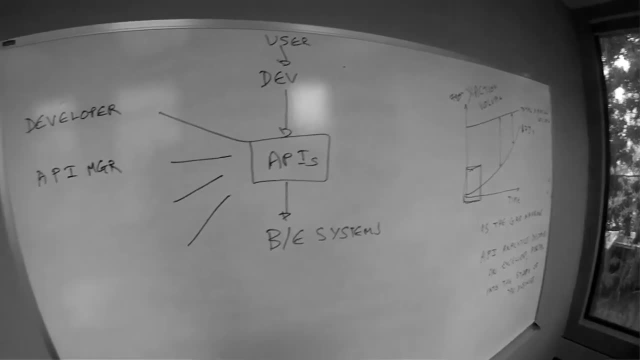 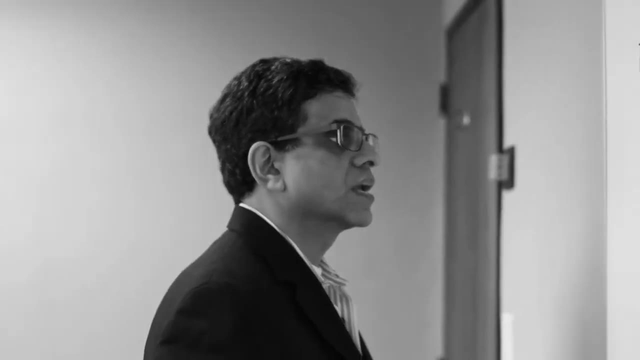 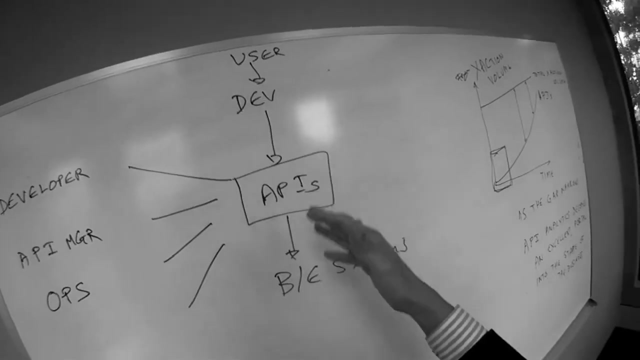 would then help demonstrate to perhaps the skeptics within the enterprise that API is not a flash in the pan but is actually a legitimate part of their business strategy. If I am an ops person, I may be interested in understanding the response time associated with those different API requests. 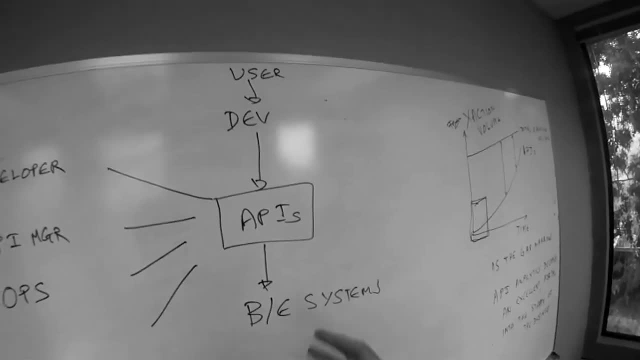 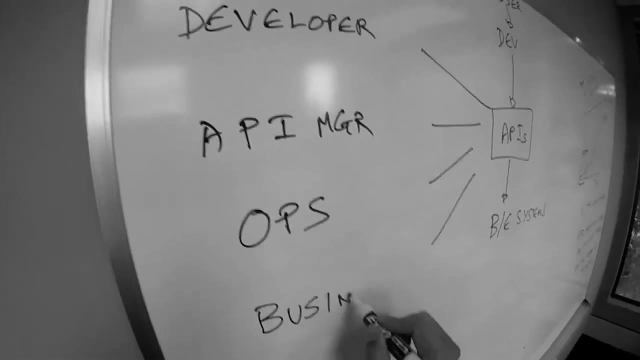 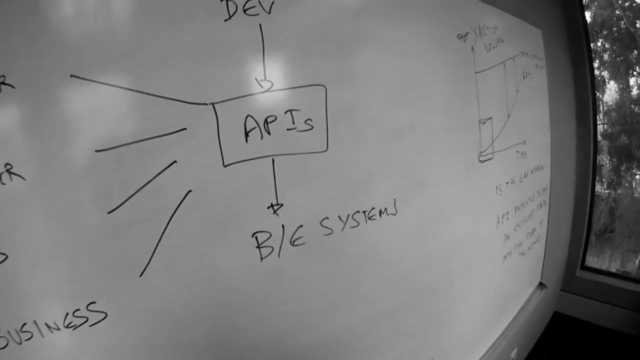 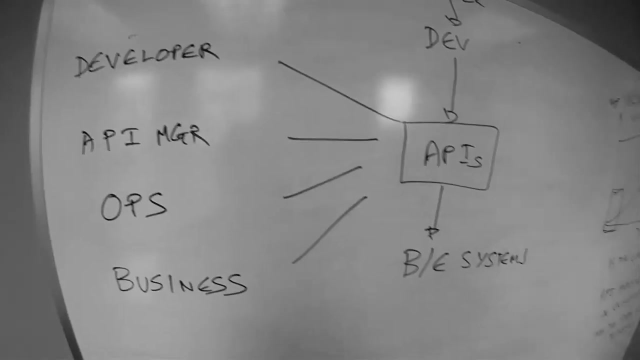 And I might want to provide some information to the API manager. If I am a business person and I am trying to figure out, how do I actually either reach the developers or how do I spend on APIs compared to some other channels, with respect to my marketing dollars or my development dollars, or even my investment dollars? I 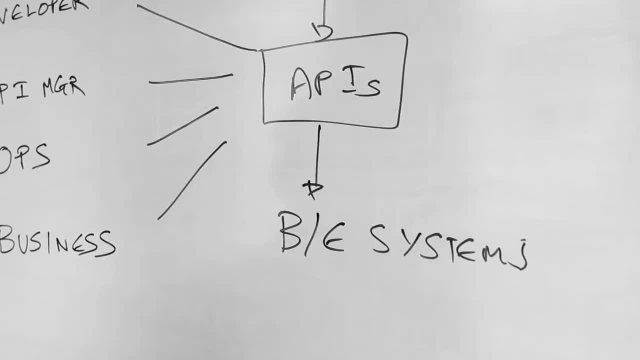 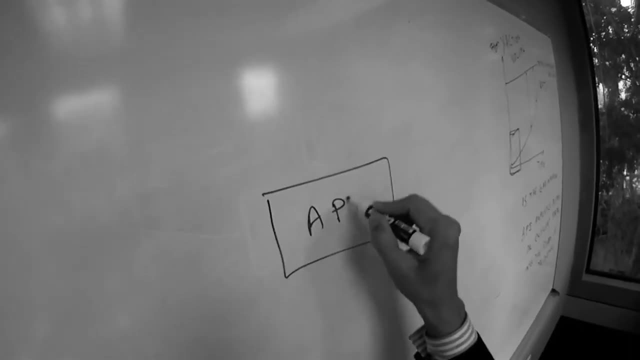 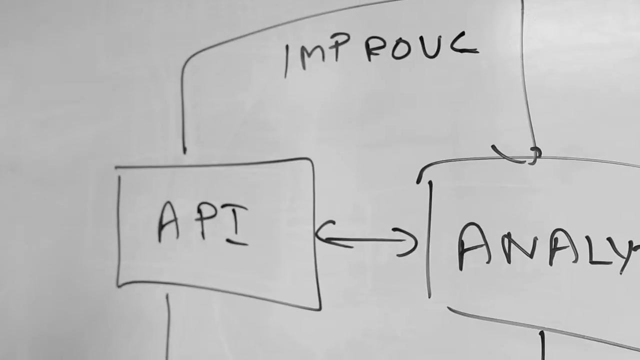 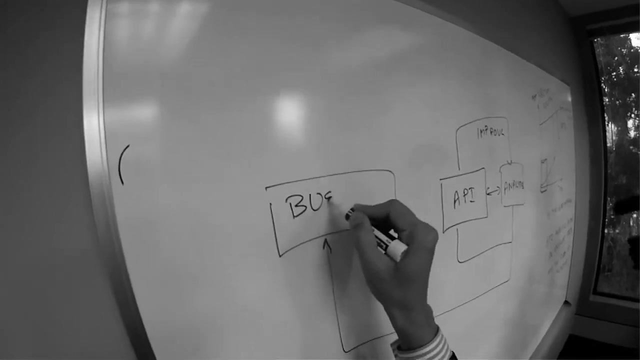 would be interested in understanding the bottom line contributions. So, as we have said, if a company is just embarking on the API journey, that analytics helps improve APIs. But analytics becomes even more important as your APIs improve because, over time, analytics 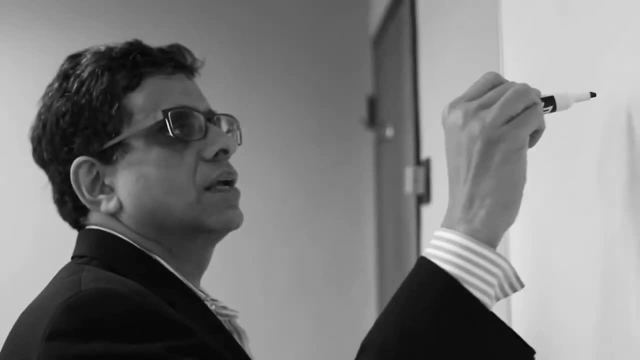 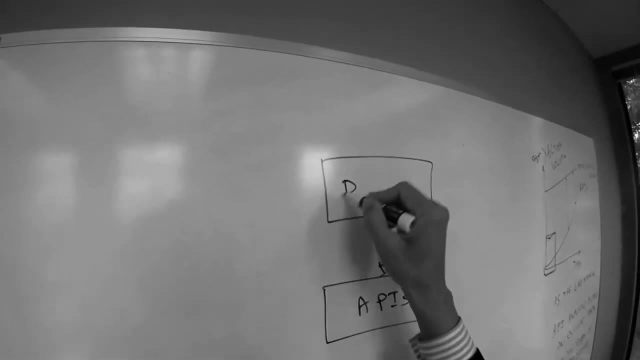 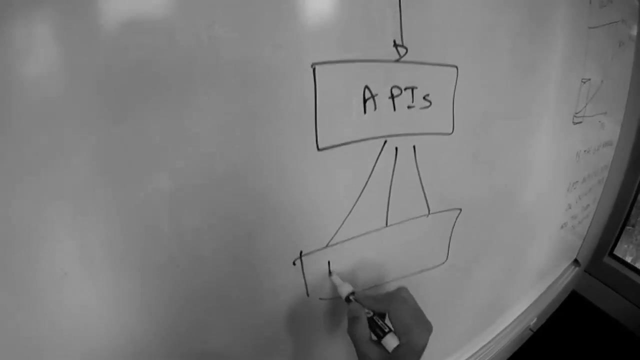 actually helps you improve your business. So, if you look at APIs, Think of Apple as a front-end solution. if you can use whale engines to run the backend services in Google, if you want to have a business that is built on the Dlatego successful. 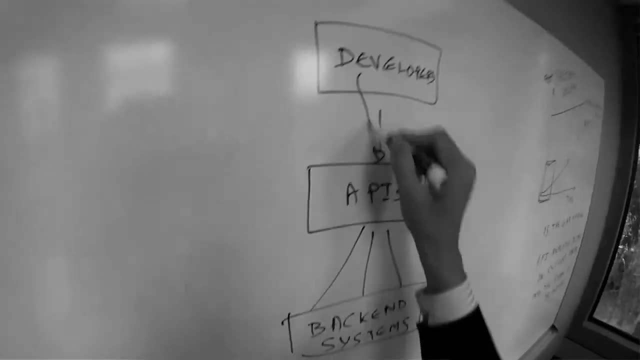 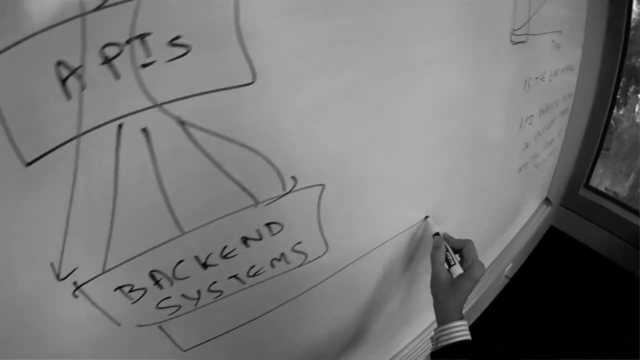 layer, What you can write about Interceptus, or how you want to write about Scrum or whatever you want to write about your automation team as the front-end bedroom, and if it works, then what you will do is implement strategies that work. Carter greedyм. 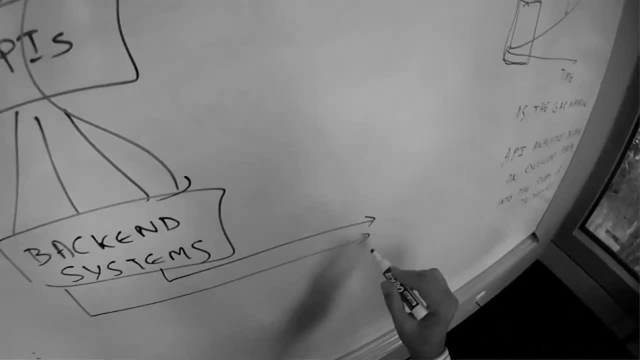 it's really time consuming and what you need to do. by the way to 2005, development has to develop really well. It's the middle of 2017 that the market shows where it writes for few days because more single anytime, and again it's a новa要ан.